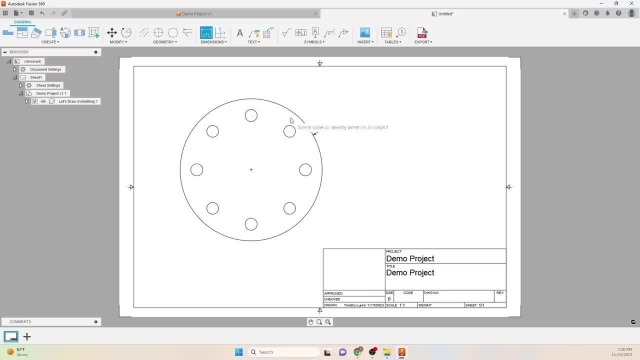 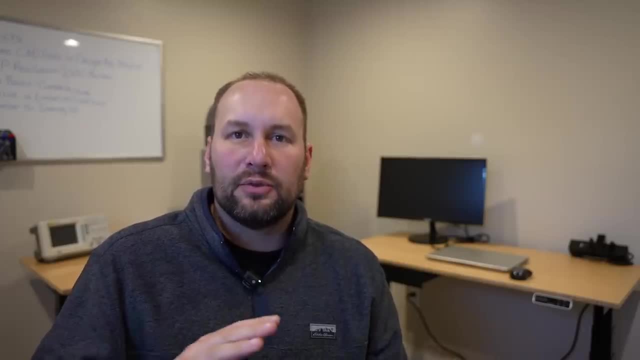 can use completely free of charge for your own personal projects. The first four are traditional CAD software and the last one is an easy-to-use drawing program that I use all the time without all the hassle of traditional CAD, so be sure to stick around for that one Now. this video is 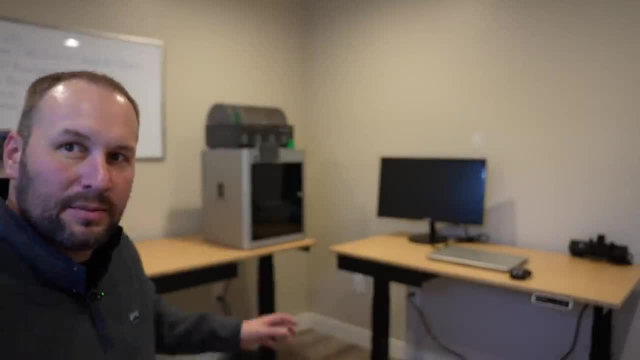 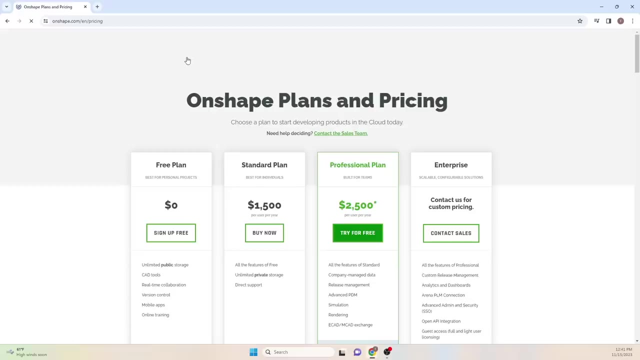 sponsored by FlexiSpot. They are the makers of these awesome desks that I have here set up in my office. More about them in a little bit. The first option we'll look at is Onshape, and they have a bunch of different plans available for corporate accounts, but their free plan. 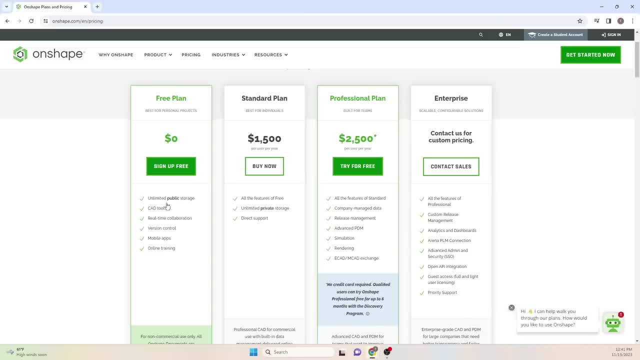 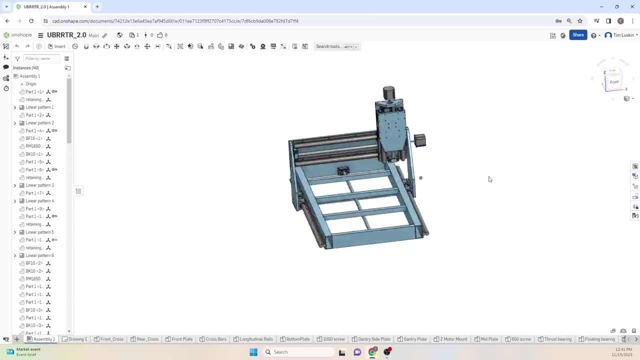 has a couple limitations. One is that all of your documents have to be publicly available, and the other one is it is for non-commercial use. This is a CNC router that I designed in Onshape. You can see how you can put a whole bunch of different parts. 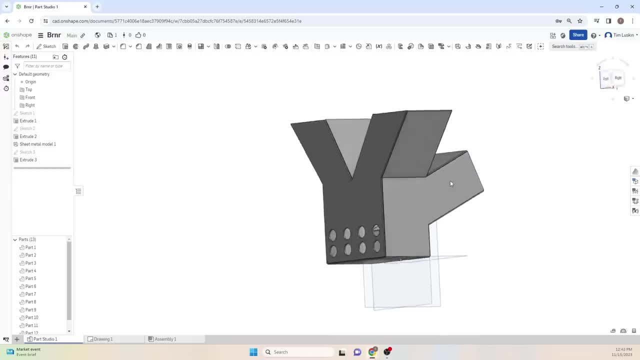 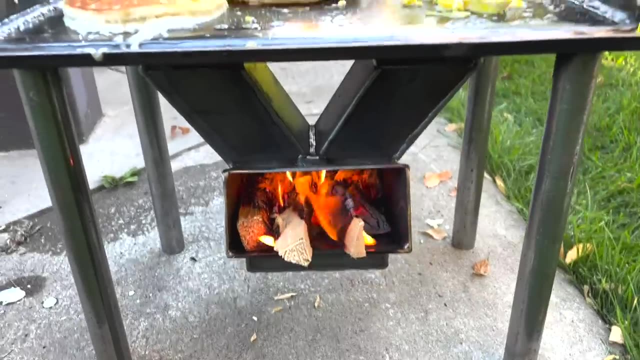 together, or something simple like this burner for a double rocket stove that I modeled up so that I could CNC cut the parts on a recent video and put that little stove together. So it's really useful to model things up. Also, this is a welding cart that I built a few years ago. 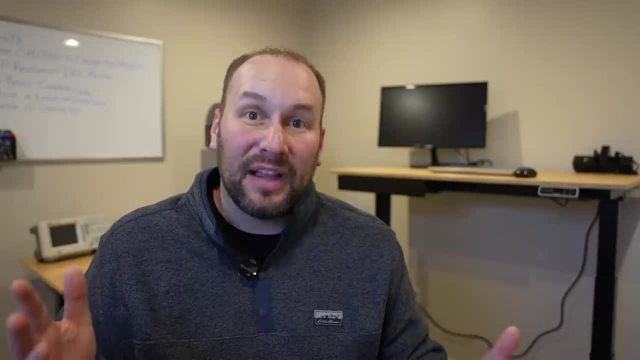 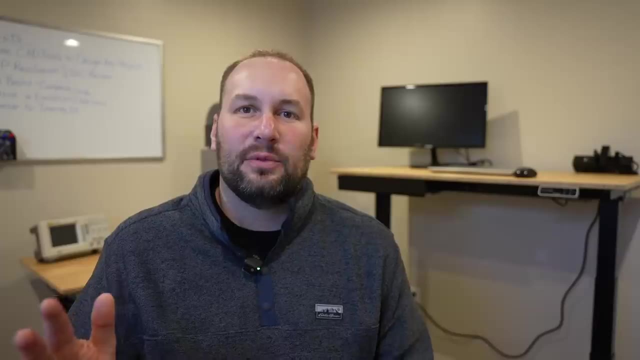 Now I will spend a little bit of time clicking around in each one to give a flavor of what you're going to be looking at, but this is not a tutorial intended to teach you how to use the Onshape. There are plenty of those available online for each one of the packages that we'll look at. 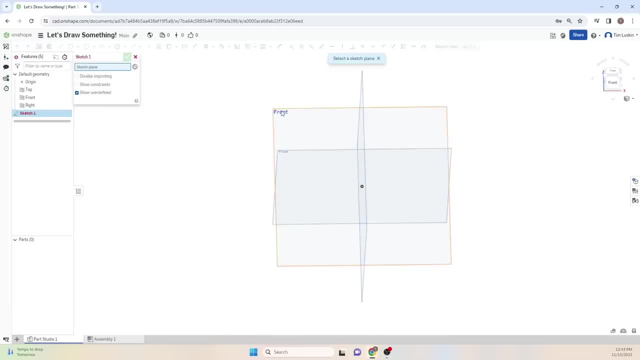 Now, Onshape doesn't have any software to download. It runs completely in a web browser, which is pretty remarkable, And I think the interface in here is pretty nice and the most intuitive of all the packages, because all of the icons- and there aren't too many- really illustrate and show what they do. So if you aren't familiar with 3D modeling, 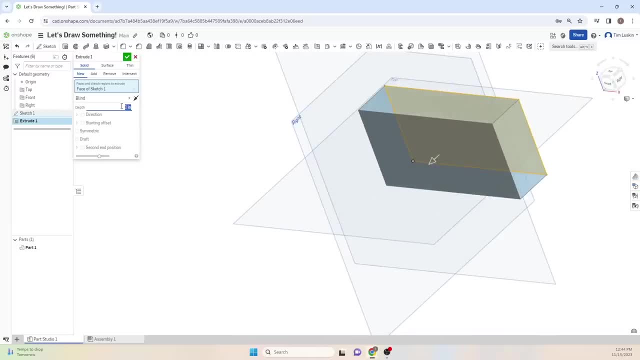 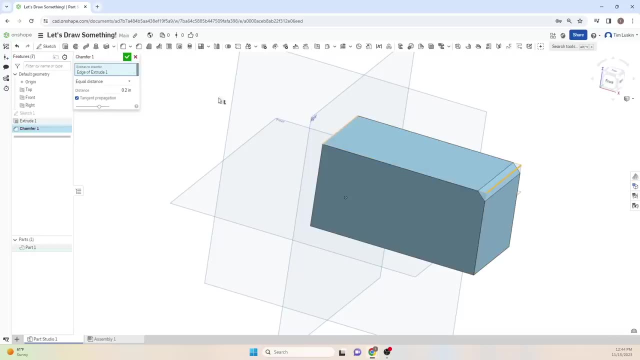 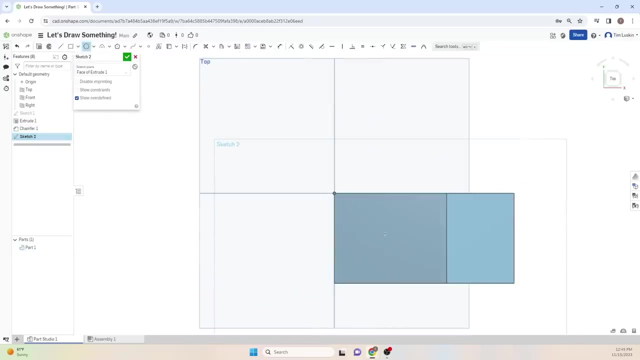 often you'll do it by starting with a two-dimensional sketch and then you'll stretch that out to extrude it into a shape, And here I made that rectangular prism and I can modify it by putting a chamfer on here, And these are standard tools that are available in most CAD systems. You can actually make a lot with simple tools like that. 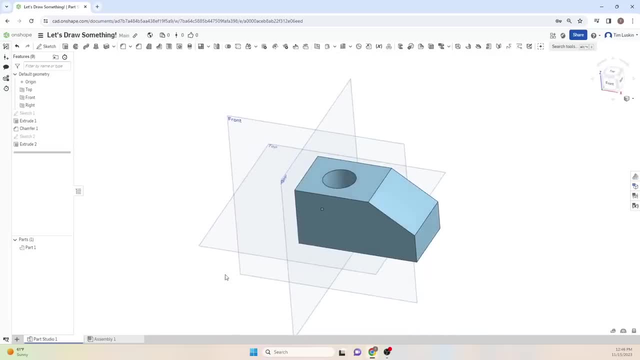 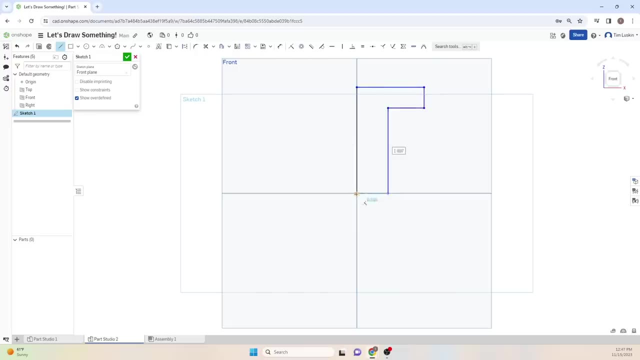 So I can add another feature here. I'm just modeling up a little block that is often used as a drafting exercise for hand drawing. Believe it or not, I actually took hand drafting classes back in school. I'll just make a little pin that comes out of the back of my pen. 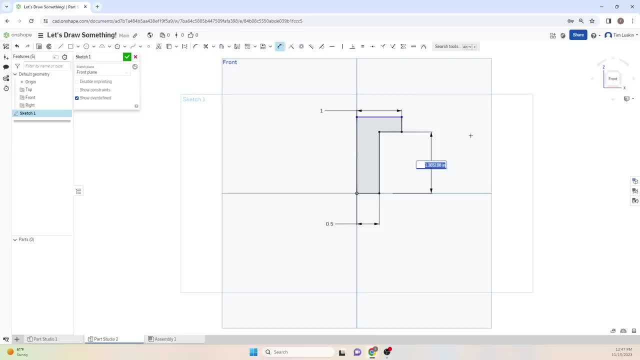 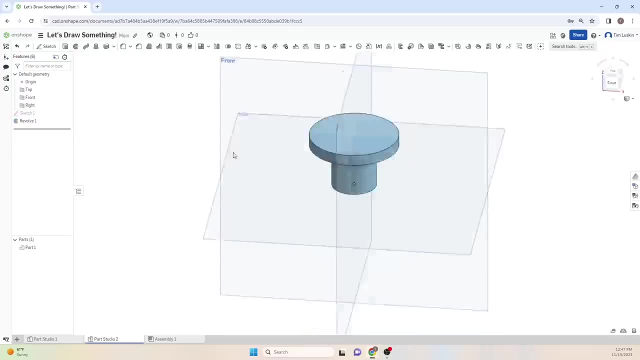 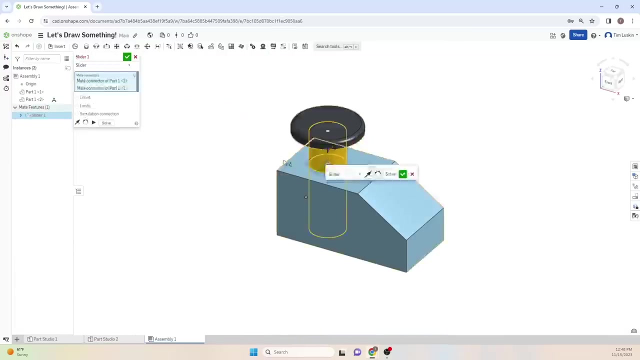 And I'm going to do this by making a sketch and revolving it around an axis rather than extruding it, And this is the other common operation that you'll do in any of these CAD systems. And while there's more advanced things you can do, those will get you a long ways. 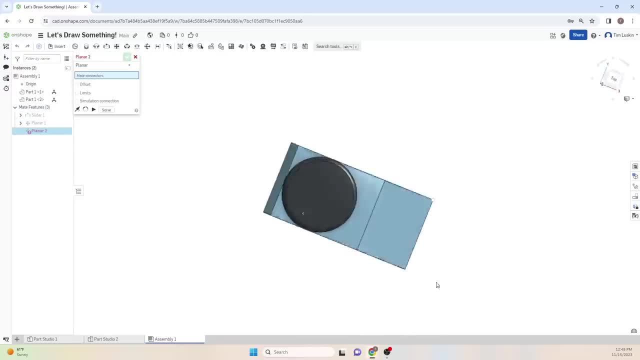 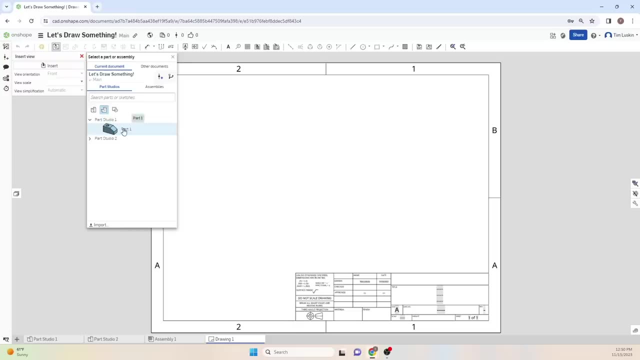 Now here in assembly mode, you can actually easily put things together and relate them and see how they move relatively to one another, which is a great feature of designing your projects in CAD. Or you can go ahead and create 2D drawings that you can use to send them to a machine shop, or even patterns to laser cut. here. 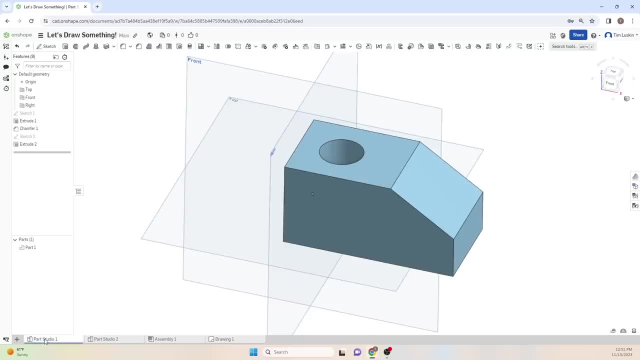 And you can do all this and export and print the drawings and everything right in the free version. You can also export the 3D geometry here to be able to CNC machine or 3D print, which I went ahead and did while I was sitting here. 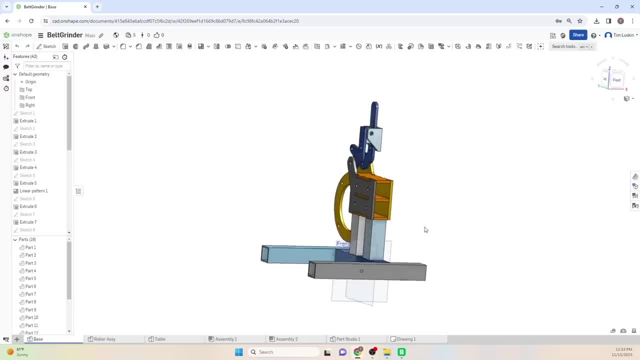 Now, these simple operations are all I use to create this whole project. Now, these simple operations are all I use to create this whole project. Now, these simple operations are all I use to create this whole project. I've used this whole belt grinder chassis in several other projects and there are some more advanced features. pretty cool for something web-based. 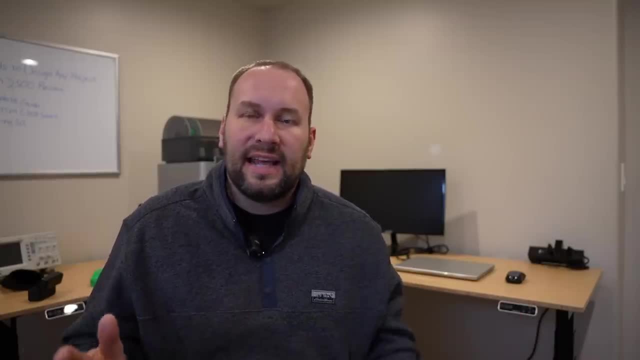 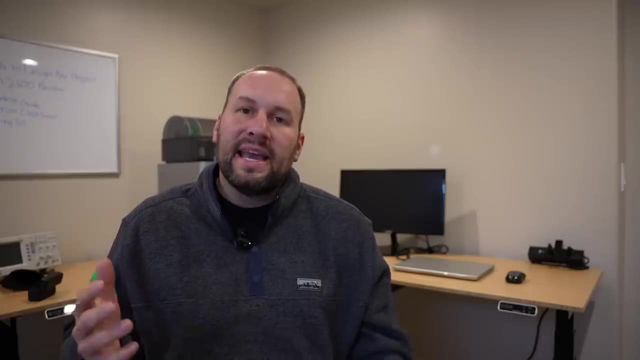 So, out of all of the options that we are looking at here today, I think Onshape is the most intuitive and user-friendly on the interface, And it's convenient that you don't have to download anything And you can access your designs and work on them from any computer or mobile device, as long as you have an internet connection. 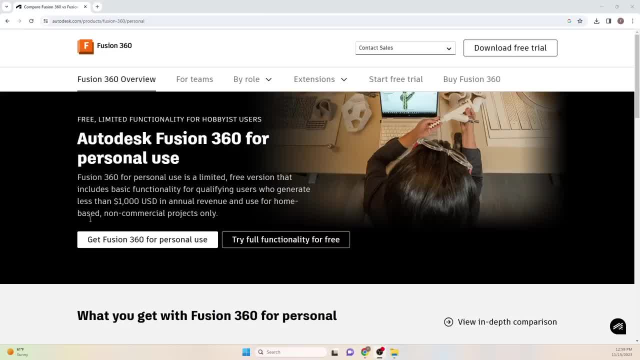 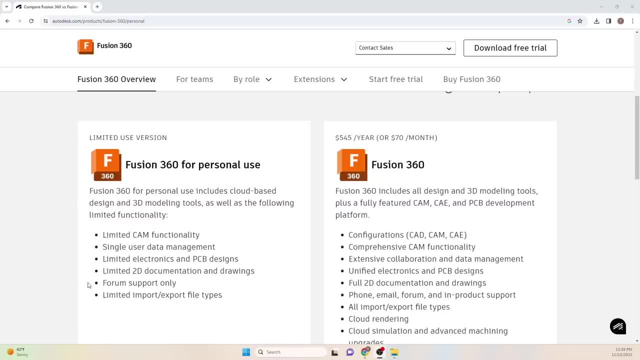 The next option we'll look at here is Autodesk's Fusion 360 for personal use. this is a pretty popular one. They've sponsored a lot of uh online content and things really got their name out there. Now this is really capable. They also have their paid version. 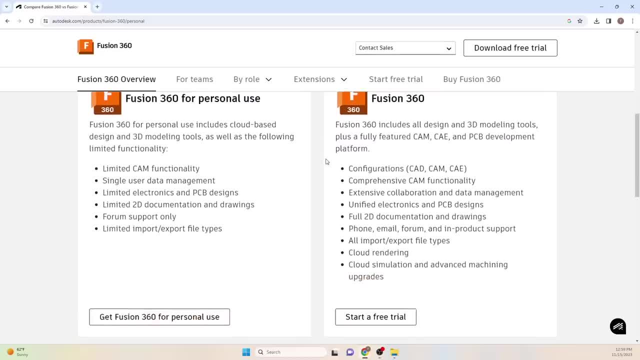 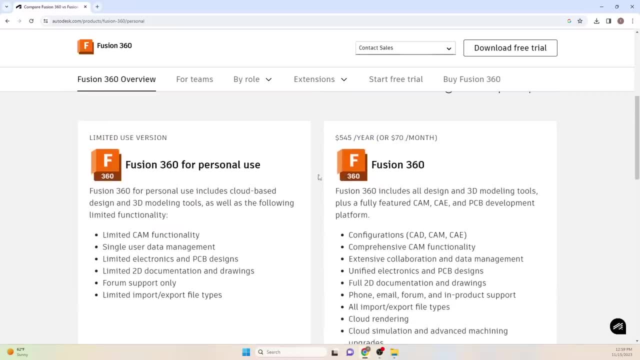 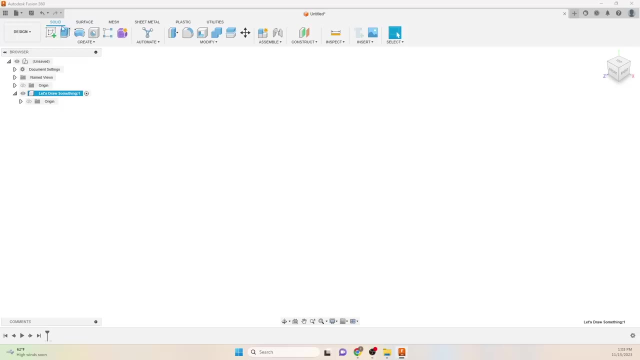 which I pay for and use for my own business here, because I think it's a lot of capability for the money on that licensing fee. So it's really good. But the personal use version is really powerful as well And I am actually using my paid subscription So hopefully I don't miss. 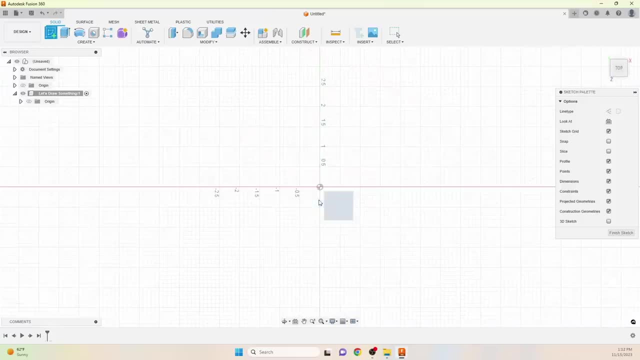 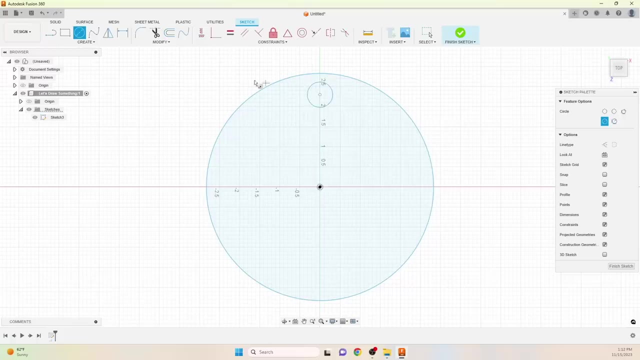 speak. If I do, let me know in the comments on what you're able to do in the personal version, but I'm pretty sure I have a good understanding of it. Now, once again, I made a sketch here, and this time I'm just going to draw up a simple flange, because I want to show you a feature that 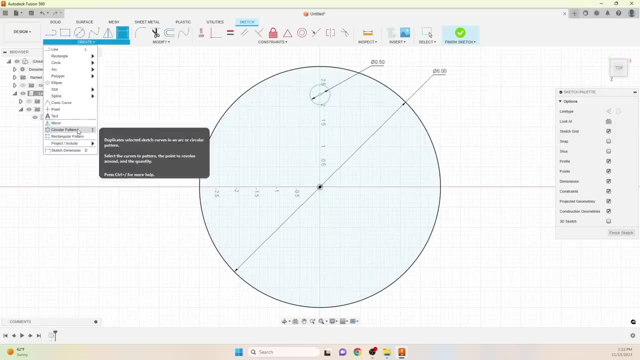 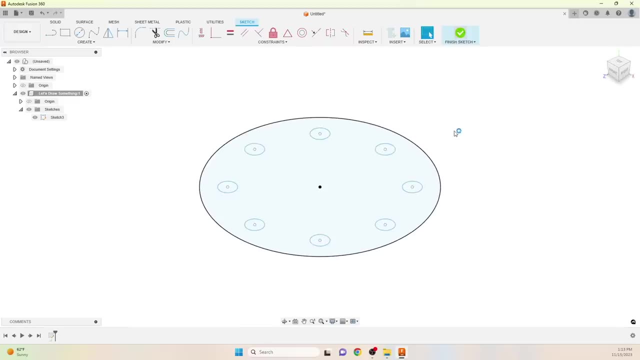 as far as I know, is only available in Autodesk Fusion 360.. So I'll just uh, add some holes here to this sketch and notice there's still light blue in the center, because I didn't fully define the position. but it'll be okay for a demonstration Now if I 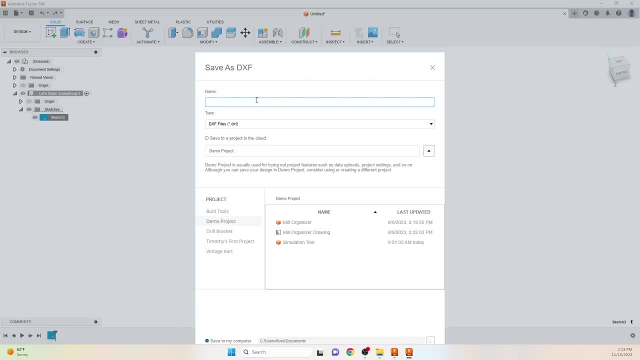 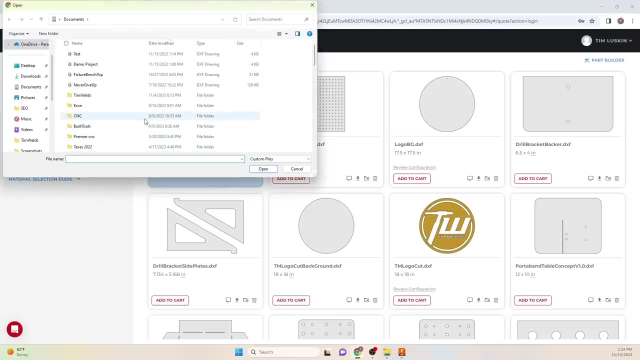 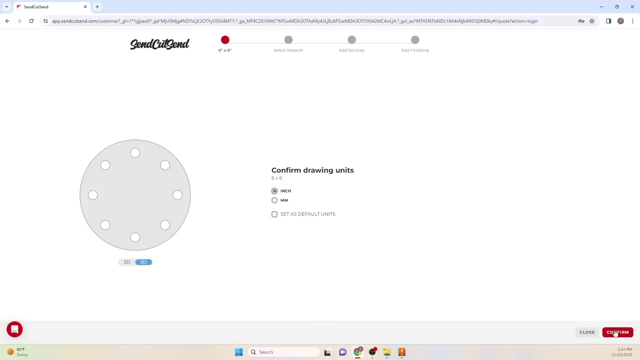 right click here on the sketch, I can save it as a DXF file to use for a laser or plasma cutting. And this is awesome because just with that thing that I drew up right there in a couple minutes, I can go ahead and upload it to SendCutSend. I don't know why every software doesn't allow you. 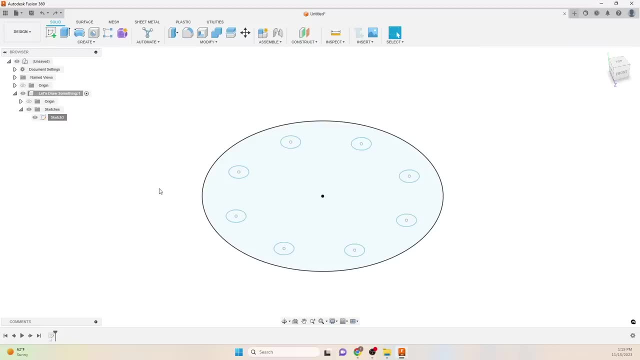 to do that, but it is really nice to be able to easily make those 2D parts. That being said, I can go ahead and extrude it to add some thickness to it, which I could then use to 3D print or put together an assembly and see how things fit together. 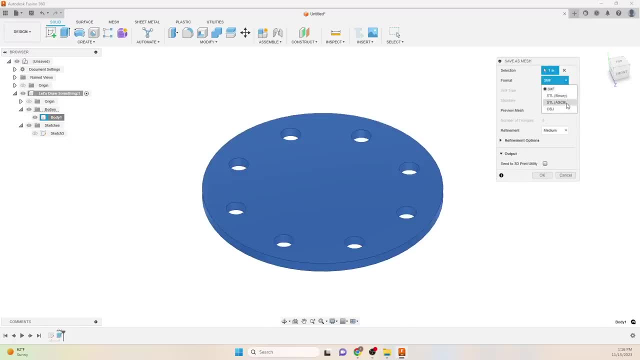 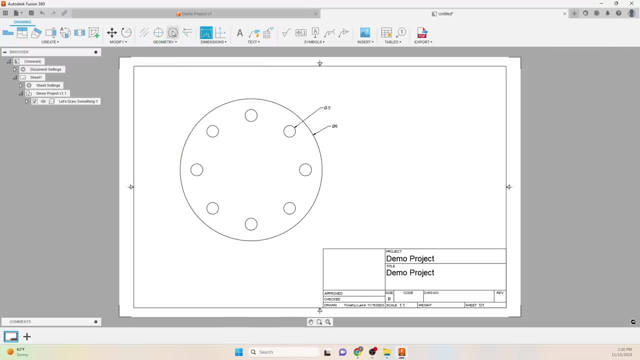 Now here is an export of a model to 3D print And, as far as I understand, this is available in the free version and you can also make technical drawings, though I believe they are limited to one sheet on the personal version and I'm not sure if they're watermarked, but 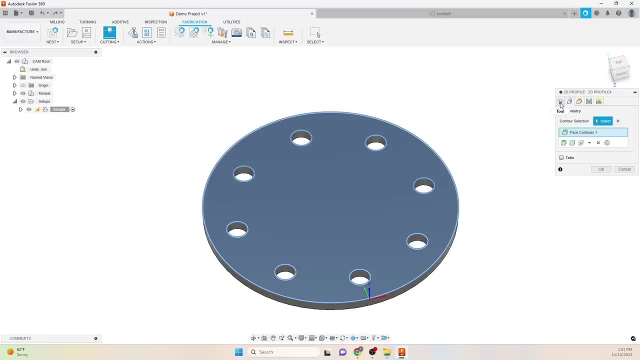 there are a few limitations on what you can export. Something that's really unique in Fusion 360 is they've integrated computer aided manufacturing, or basically programming for machine tools, here. So So what I'm doing on the screen is I'm actually creating a program to be able to CNC plasma. 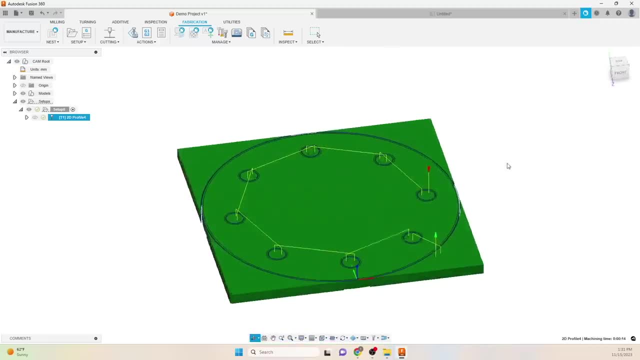 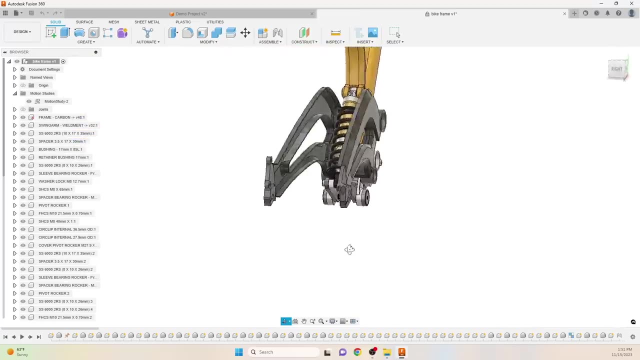 cut this right in the same software. I can export the G code right out of here and cut it out. Here is one of their example assemblies So you can see there are a lot of different components in there. The way that they handle assemblies is a little bit different in Fusion. 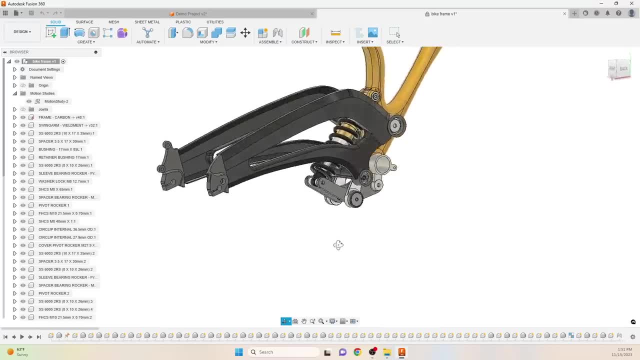 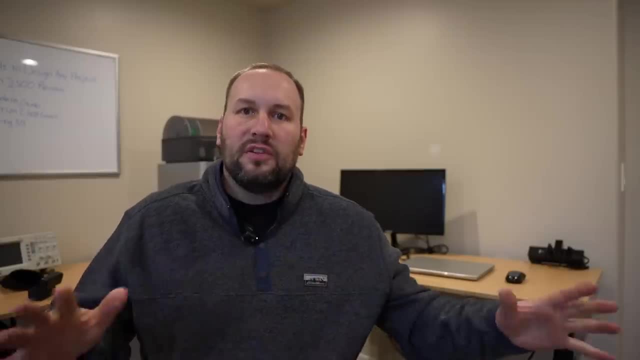 360 than in most of the CAD packages I've used, where each of the components goes into another component and you have to create a hierarchy. but it works Now from a full workflow perspective, I really think that Fusion 360 has it figured out. You know they. 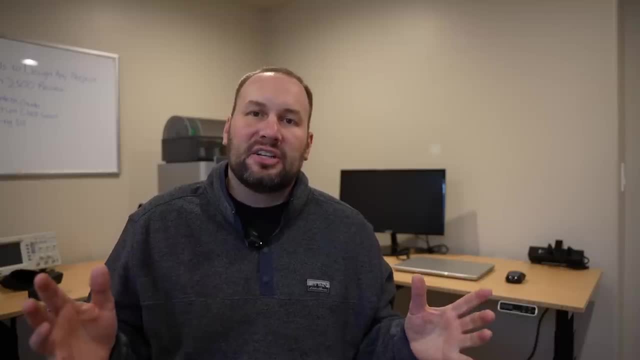 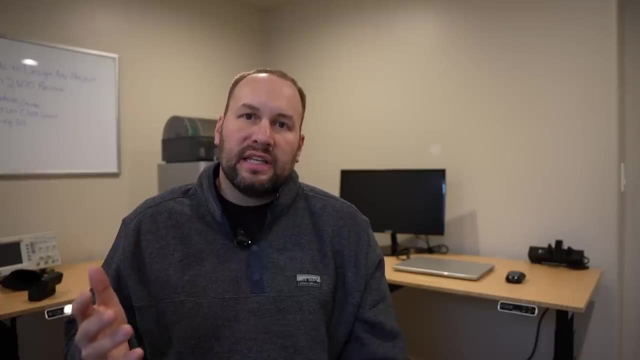 have everything from design, drafting, manufacturing and what I think they really hit very well as the price point for early and small businesses, When you do move beyond the free version into the paid tier, which I do pay for it because I get a lot of value out of it. Let's take a minute and talk about our video sponsor. And yeah, that's done. All right, Thanks, let's move on. All right, right now I'm reeling a little bit beyond UI, so I want to thank you guys for joining me today My question and I'm gonna conclude everything here and that's. 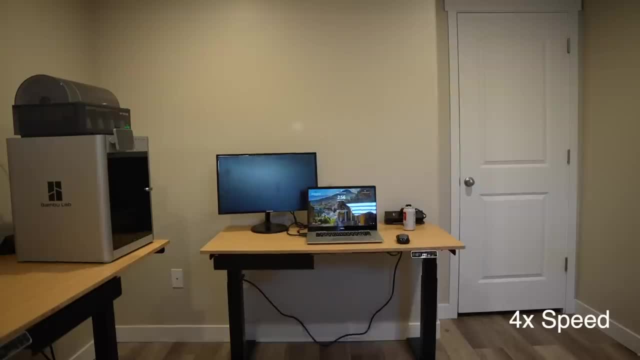 oh, yes, c'mon. obviously there's going to be a little conclusion in the future, but for it's not going to be that short. So thanks, as always, and if you all are in office sponsor and I'll show you these Flexispot E7 desks that I have in my office that go down below two. 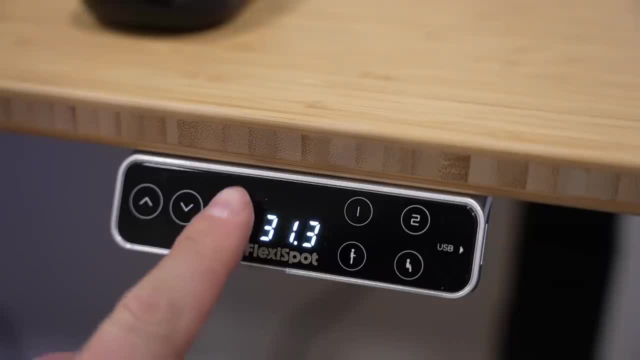 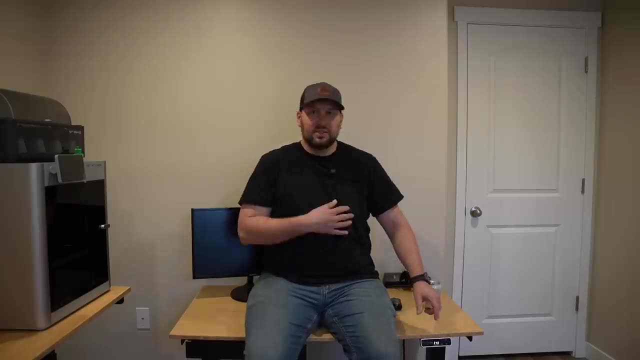 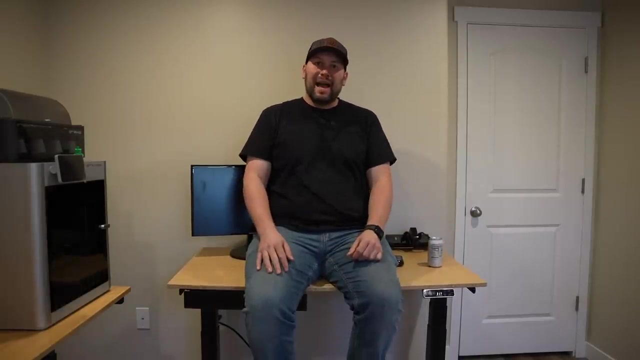 feet and rise up above four feet. That's a big range. You simply press a button to change the height and you can lock in four different presets. These things are built strong and sturdy. It's made out of thick carbon steel and it has dual motors with a 350 pound capacity. Now my computer. 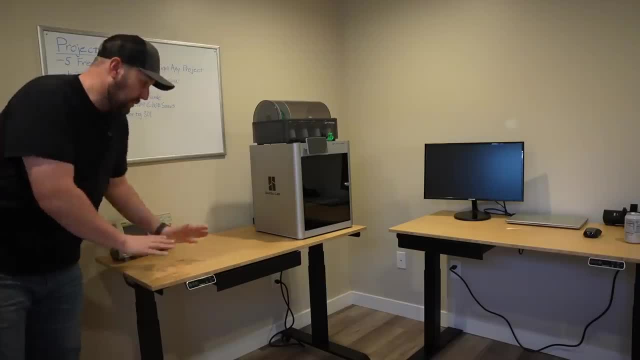 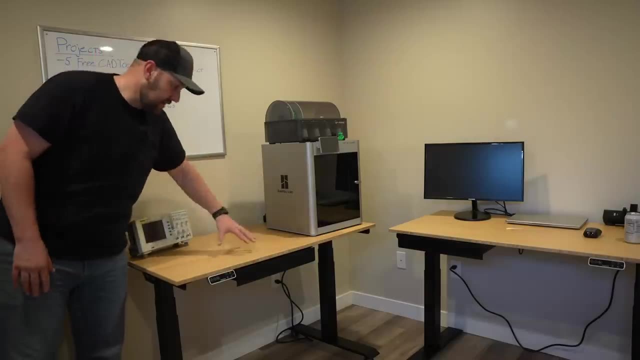 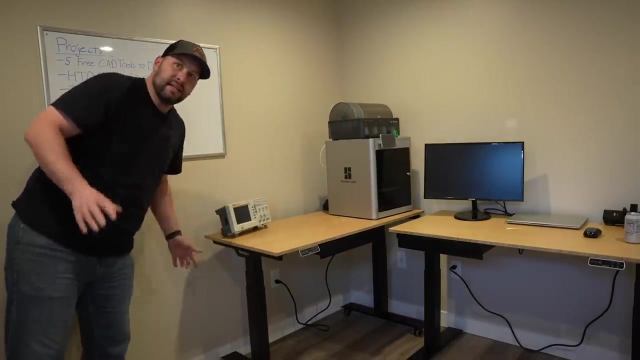 desk is fixed in place just on the feet, but I put wheels. They have some wheels available. I put those on this desk for project stuff. so I have my 3D printer there, room to do some breadboarding or electronic prototyping and things like that, right there and I can tuck it up tight if I want. 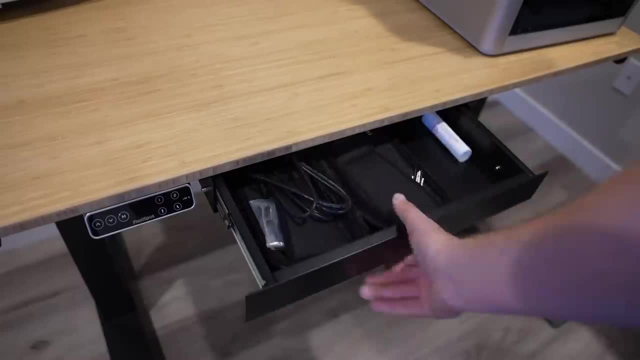 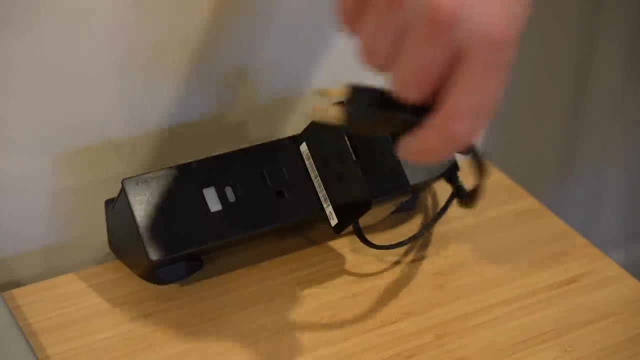 the rest of the room open or move it over. Now I have some modular accessories on here. There are drawers on each one to hold some of my items, power strips to plug everything in and USB charging, and as well as a cable management tray to keep everything neat and tidy and hold everything. 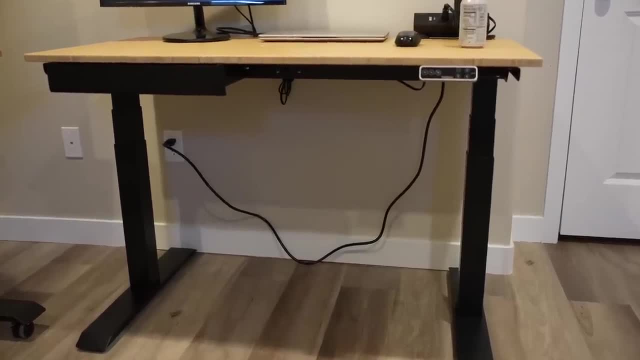 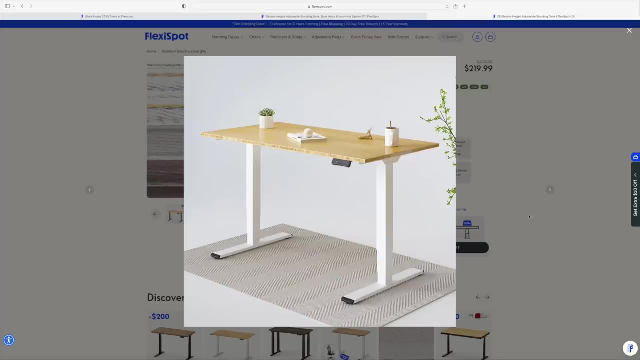 out of the way Now. I like just having one cord coming down off the desks, and they have a whole ton of other accessories available on their website. You can find anything you'd want. They also have some less expensive options, like their E5, coming in around $200, and their E2,. 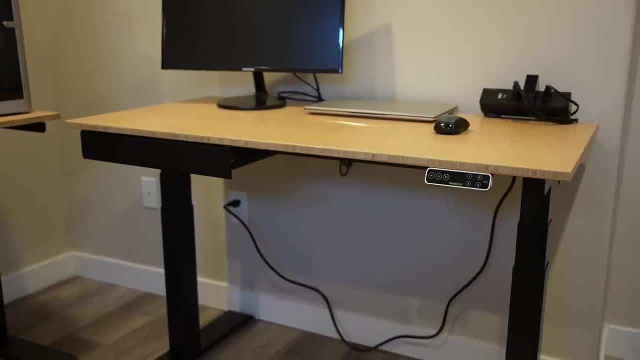 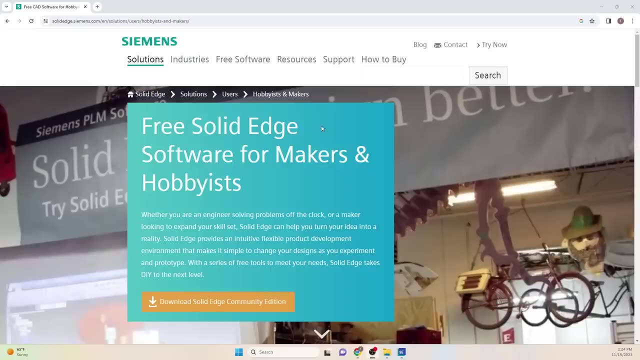 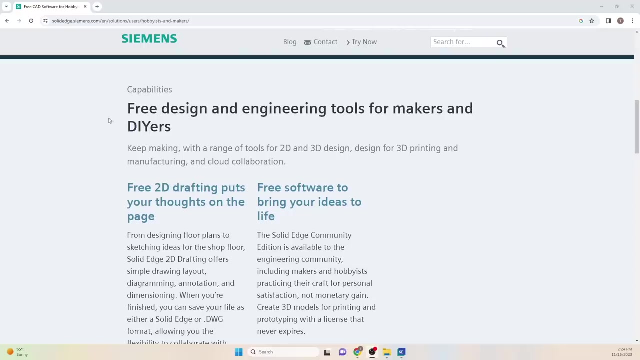 which can be completely set up for under $200.. These desks have a 30-day hassle-free return policy as well as a 15-year warranty. The next package we'll look at is Solid Edge for makers and hobbyists. Now, this is their personal edition, and I didn't even know that this existed. 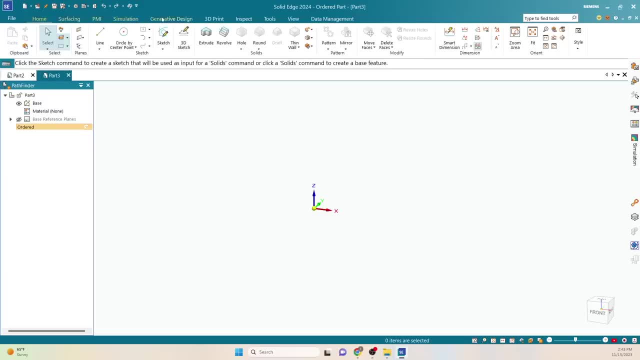 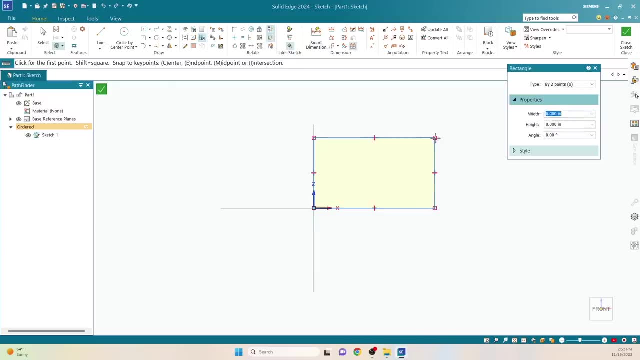 but it is really powerful and capable. but it's not for commercial use and there are some limitations on some of the features. But once again in here I can open it up and perform all my simple modeling tasks. Notice at the top just how many commands there are available. 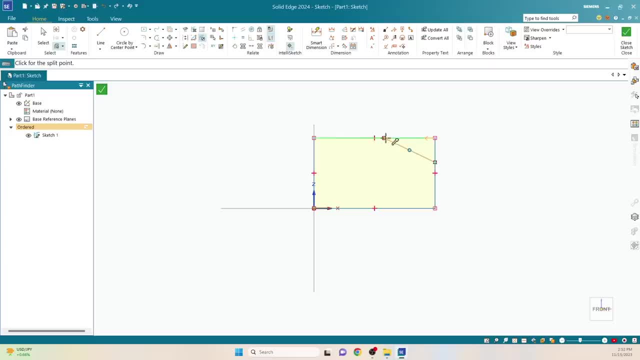 to me. I can open it up and see how many commands there are available to me. I can open it up and see how many commands there are available to you all the time. I think that makes it a little bit less user-friendly, honestly, And this is the only package that lagged a little bit on my computer. 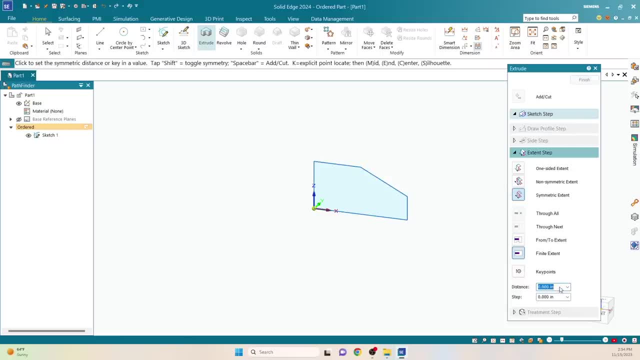 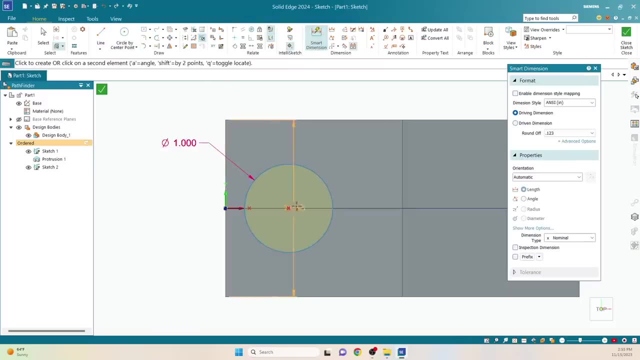 It's not a brand new computer, but it has pretty decent horsepower, so I was kind of surprised. Now there is a dialog box that walks you through creating each feature here. I won't spend a lot of time on that, but it does give a lot of control. However, it does take a little bit longer to. 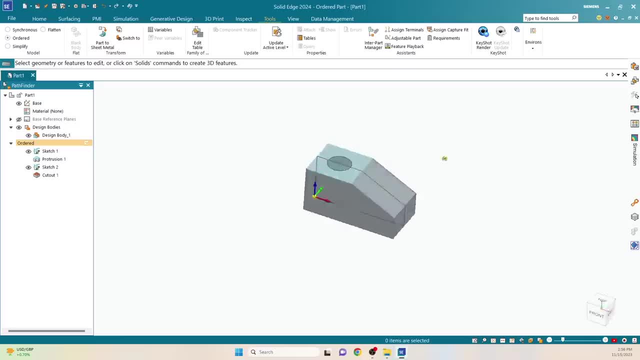 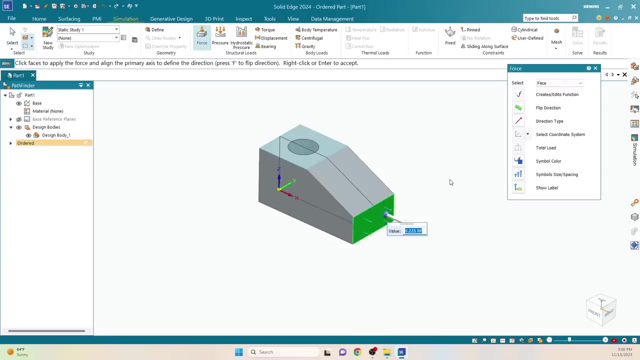 actually perform each operation. The part files you create can't move between the community edition and a paid edition of Solid Edge, so you're not able to send them off or anything there, and drawings are watermarked. So something I want to show you that I was pretty impressed with is the amount of analysis and simulation. 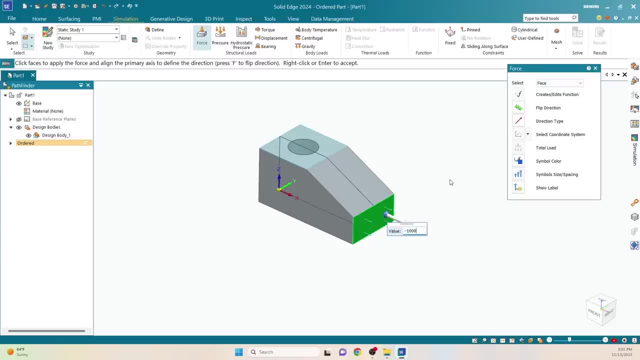 capability here in the free version Now it is somewhat limited, but you can run some structural analysis and that's pretty cool. So I defined a force here on the front face, as though something is pushing on this, and it is held in place with a pin to be able to analyze this structurally and we can get an idea of how it performs. 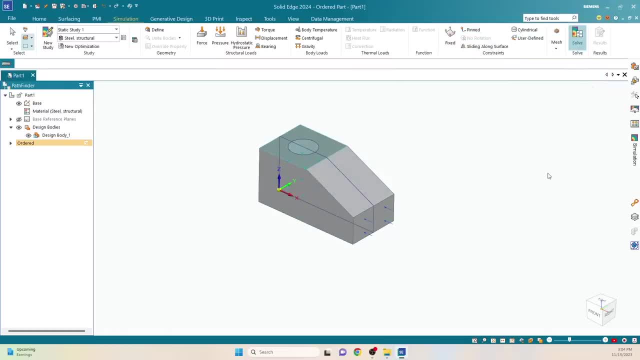 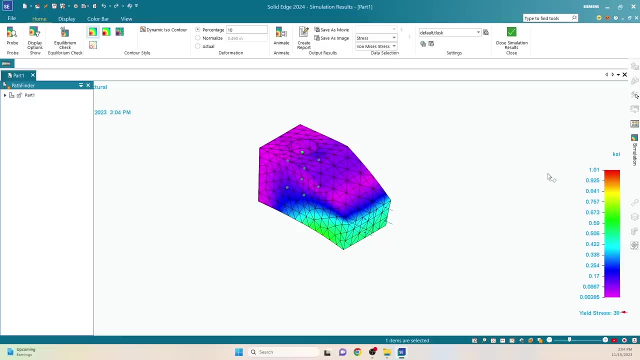 It will solve right here in the computer. Now this is a small model and it's relatively simple. And keep in mind, there's a lot of nuance to running an analysis like this and so you want to be a bit careful if you are new to structural analysis. But to be able to start and play around with it in a free version is pretty cool. 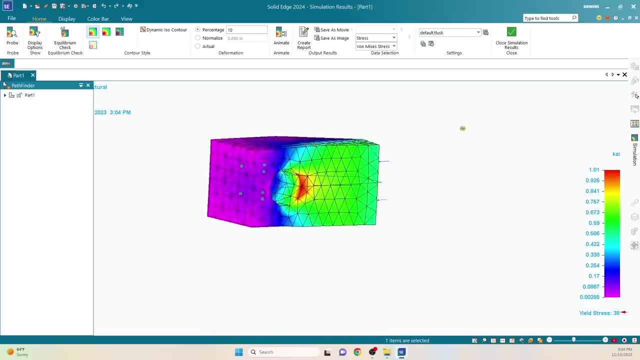 So you can see right here, based on the load applied, that is the stress that I'd expect to see right there around the front face, but you can see how it will deform- Of course that's exaggerated there for visualization purposes- as well as how the stress is distributed. So I thought that was pretty neat. 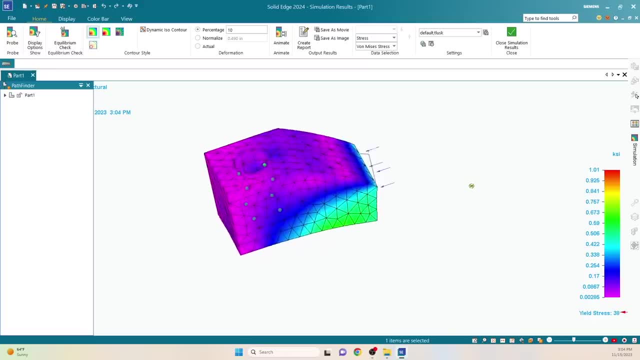 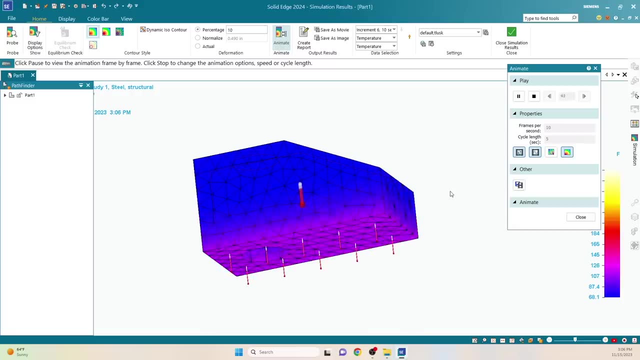 and that could be pretty useful to start getting your feet wet with some analysis and get an idea of your designs. But again, proceed with caution here. Now this is a thermal simulation showing what happens when the blood, the block, is cool, That's what it means when it's blue and you put it on a hot plate. 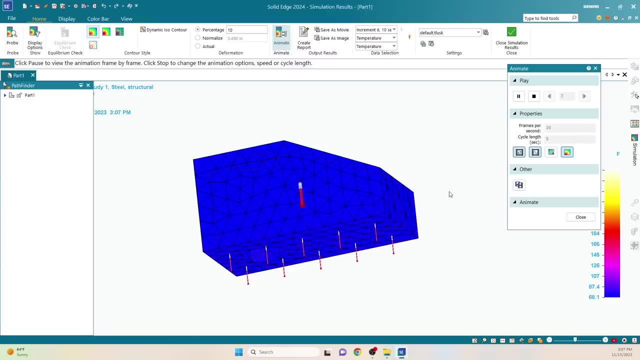 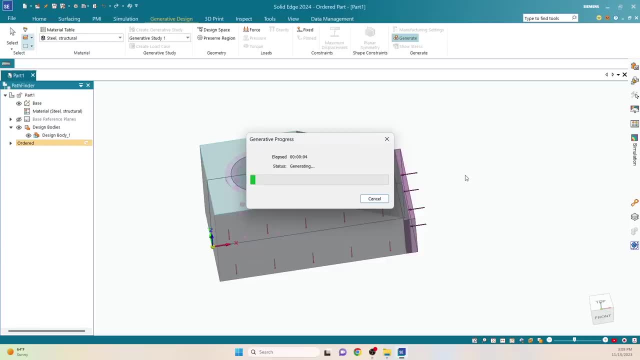 You can see how that heat progresses through the block over time. So this could be pretty useful if you wanted to look at a heat sink or something else like that. Also, it can run some generative design. Basically, it will tell you where material should be. 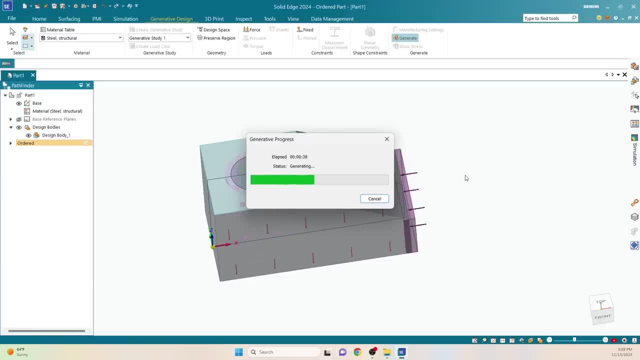 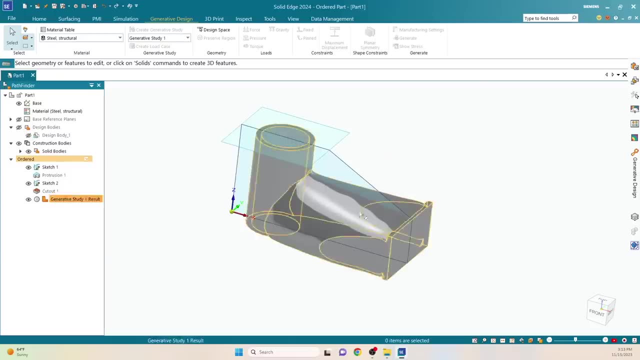 to be able to handle the loads that you define. So I used the same situation that I did in the first case, with that force on the front face And it ran through to show me where I should have material if I want to have a more efficient part. 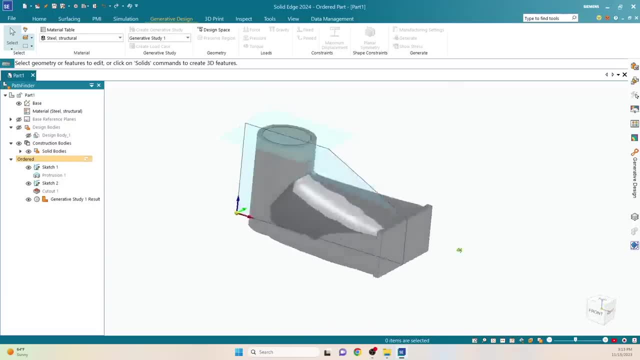 So I ended up with something like this to be able to handle that load. So this is a very simple example, but you can see how this would be really useful on something more complicated, to be able to potentially design a better structure. I don't have a lot of experience with Solid Edge. I just downloaded it to try out. 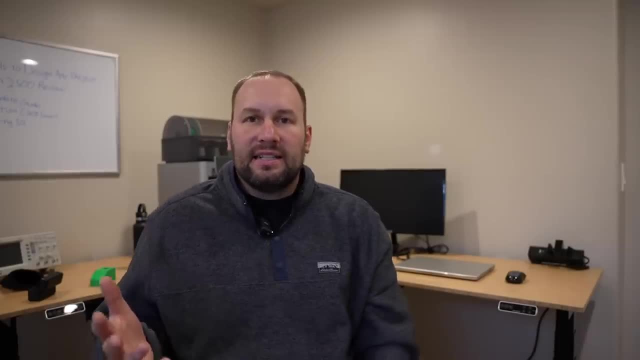 because I didn't even know they had this Community Edition until I was working on this video and I happened to cross it. But I think it's really powerful. You know, they have some of the simulation and generative design features built in there. 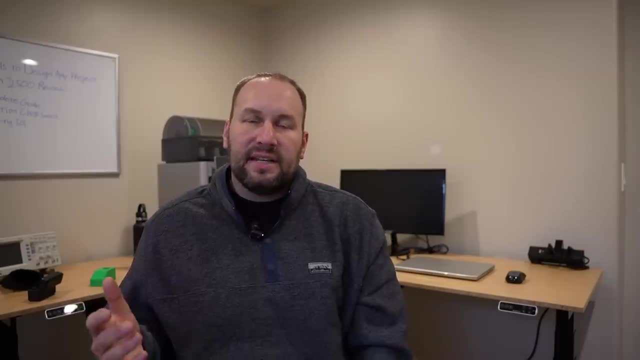 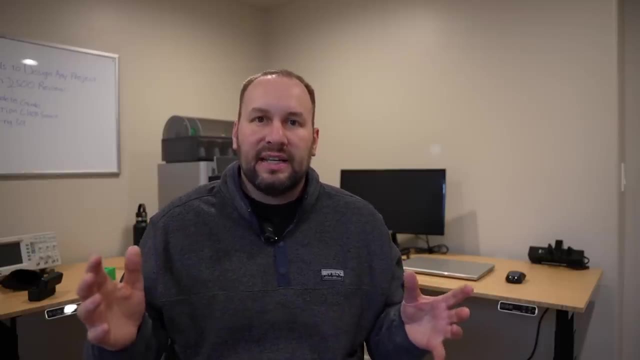 That was really cool to see that, even though it's limited, there is some of that capability in the free version. So if you want to get into some of that more advanced engineering and look at some of the other features, I think it's really powerful. 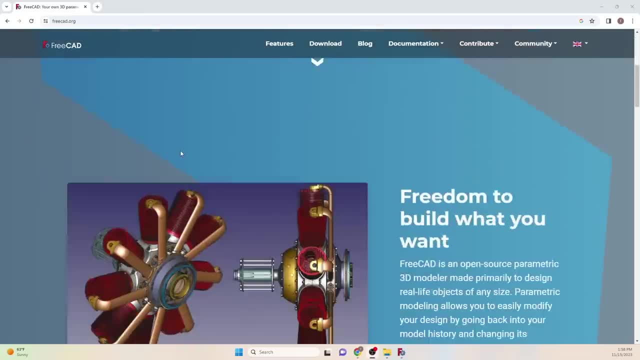 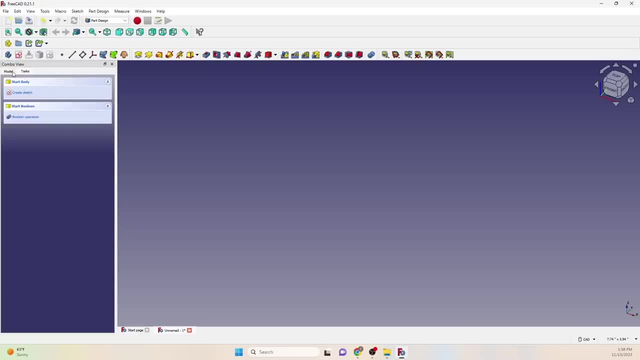 Next we'll take a look at FreeCAD, and this is the only traditional CAD package we're looking at here today. that is completely full version, no restrictions, freely available Here in the interface. you can see it does just look a little bit more dated. 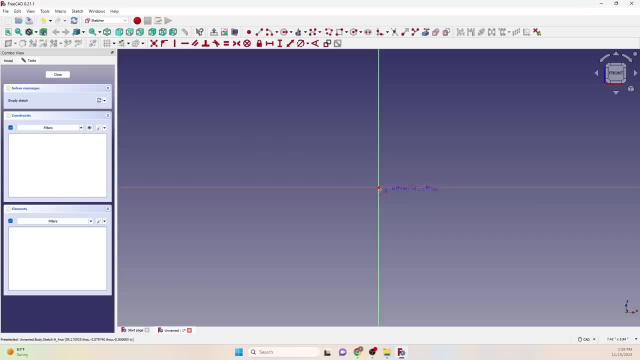 and there is a little bit more going on, So it takes some more cognitive load to actually draw and model things up than the other packages that we use. So I'm drawing up that similar block that we made a couple of times here and, as I put dimensions on here, watch if I just go around and use that same block. 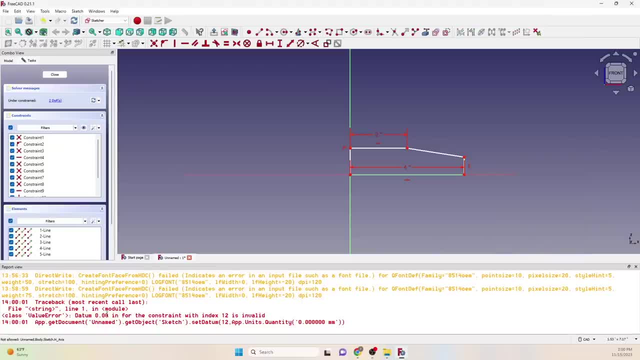 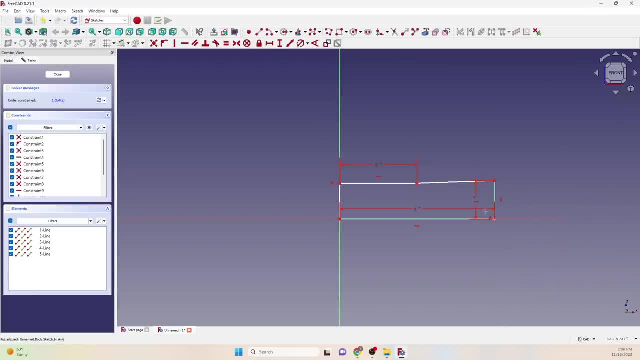 and the same dimension tool, like I did in all the others. Bam, There's a bunch of yellow and red text in my face, a bunch of computer code, And that's because you actually have to select different dimension tools for each type of dimension. 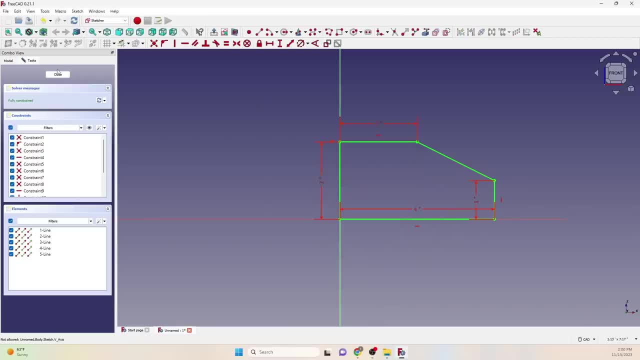 to be able to do it right Now. this is actually a pretty robust way to do things, but it is less intuitive, and so it just takes a little bit more thought as you go, And I'll tell you if you're doing much modeling, all those extra little clicks. 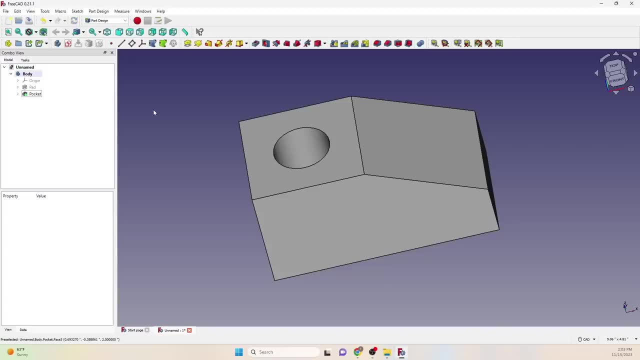 and also the extra thought that you have to put in and the energy that that draws from you. if you don't have to do that, I don't see why do it. That being said, it still works, and to be able to have this much capability available completely free. 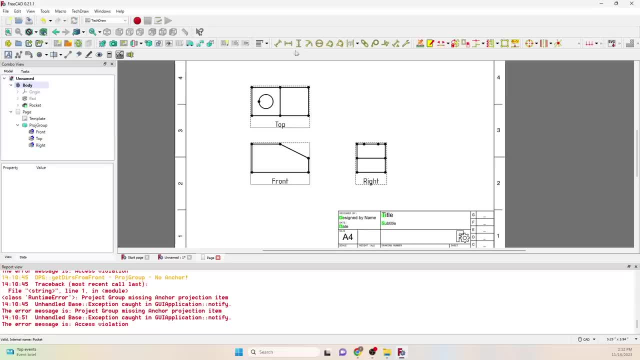 also you can create your drawings just like before When you go to put in views and dimensions and things. it's similar. You have to put a little bit more thought into how you're actually running the commands, But I think if I used it for a while, 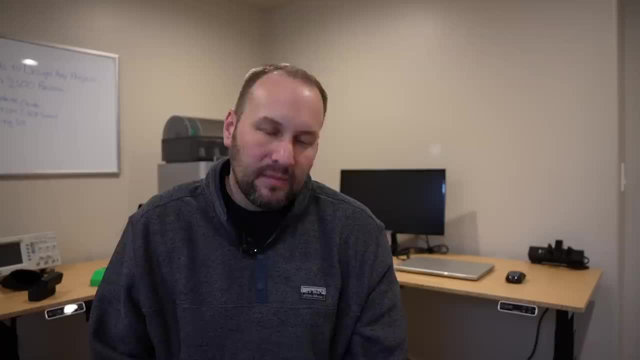 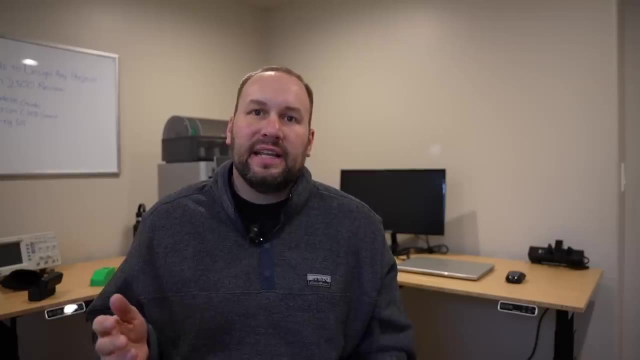 I'd get pretty accustomed to doing that Now. FreeCAD is quite powerful, but I just think it's so clunky- And that's typical of a lot of free and open source type softwares- is they just aren't quite as intuitive and user friendly. 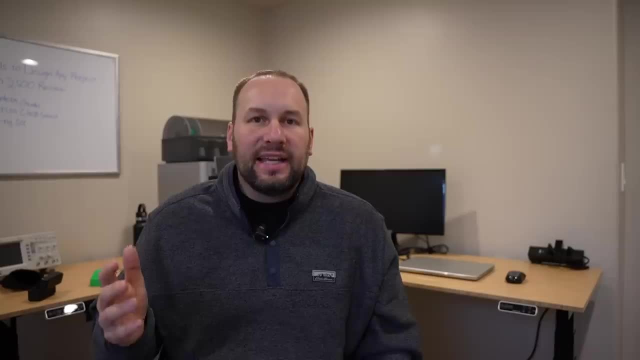 So I think that if you want a FreeCAD package with no strings attached you can use for commercial use, for your business and you're willing to go through that learning curve, it could be a great option for that. Or if you're a programmer, and you want to put in the time to code some extra features, then you can totally modify it, more so than some of the other packages. That being said, for most of us I don't think it's worth the extra hassle to use, compared to some of these other commercially supported options. 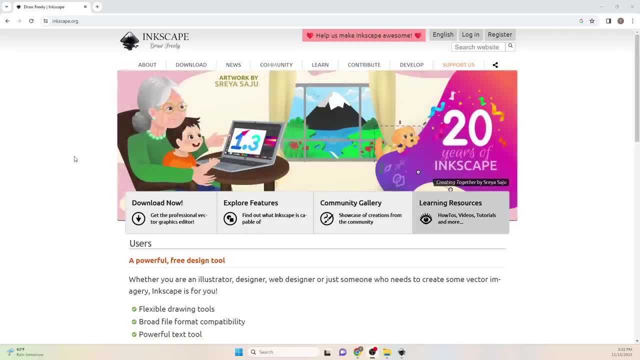 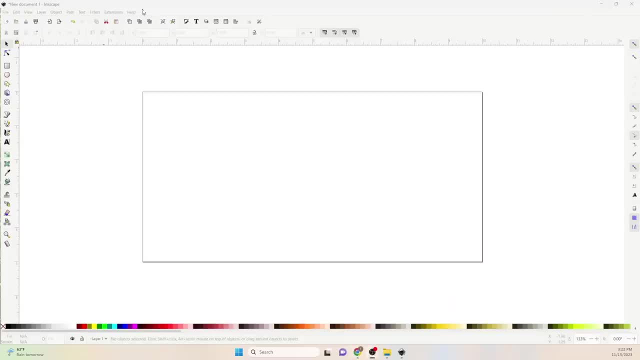 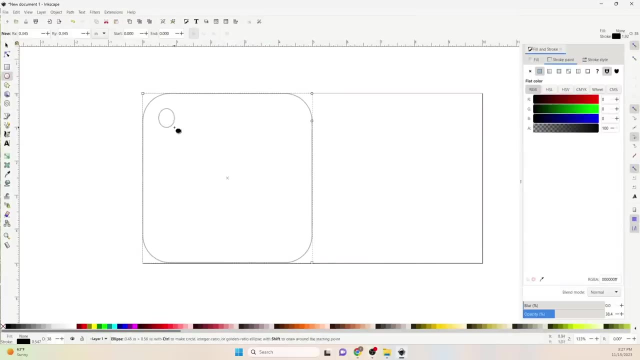 Now, the final option I'm going to show you is a drawing software, and if all this CAD has you overwhelmed, this might be a breath of fresh air. So this is Inkscape, and it is a completely free drawing software similar to like the old CorelDRAW or others out there. 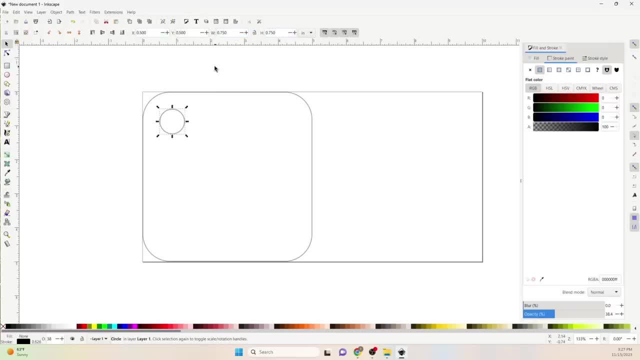 And you can actually use it to design mechanical parts, because I can type in dimensions and positions for everything like this and then use it to export things. It's also great for artistic signage and whatnot, but you can see just that fast.